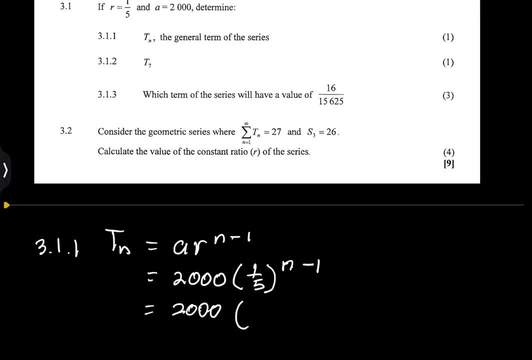 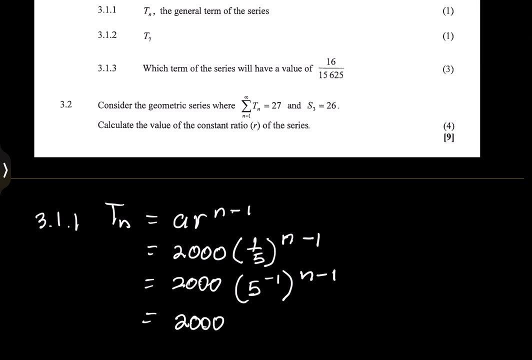 and say, well, this is going to be two thousand, okay, and remember that one over five is the same as saying five uh to the power, minus one, uh n minus one. so what you can then do is say, well, this is two thousand, okay, now, uh, of course, these are exponents, and in this case we are raising one. 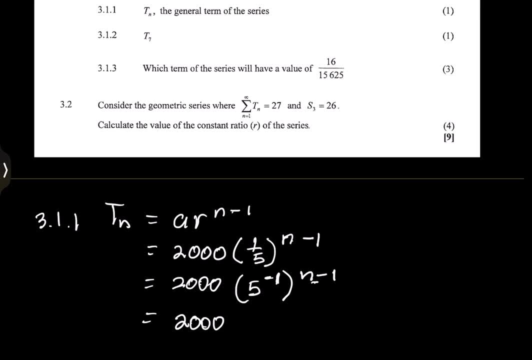 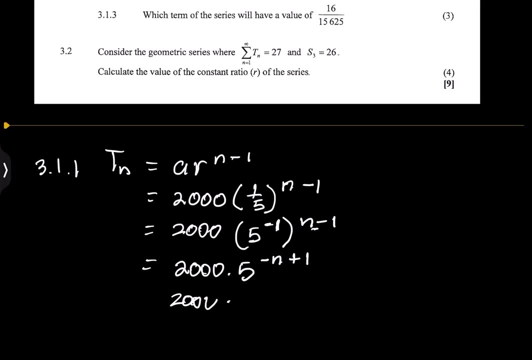 exponent with something which is on the outside. so we're going to multiply in there. so this is going to be times five. this is going to be minus n plus one. now, remember that minus n plus one. we can rewrite that as two thousand multiplied by five, to the power minus n or exponent minus n. 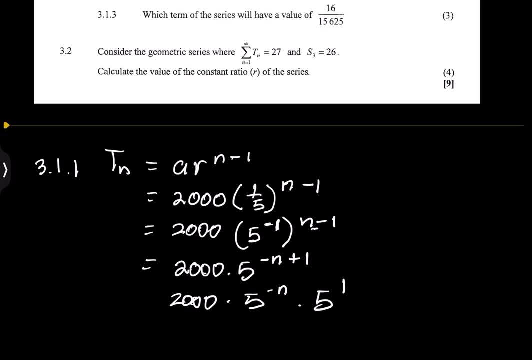 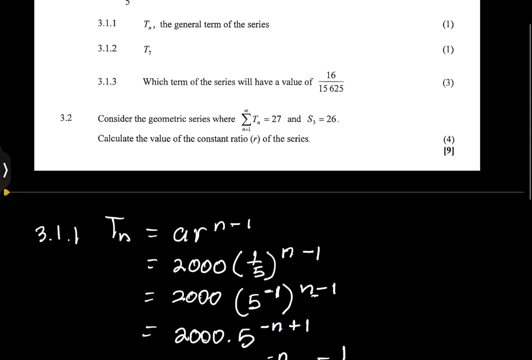 okay, multiplied by five. to the power my, to the power one, right? so in this case i remember we've got five multiplied by two thousand and that should give us ten thousand, okay, multiplied by five minus n. so this would be probably the most simplified function form in which you can write that. okay, i hope that makes sense. all right, now the next question. 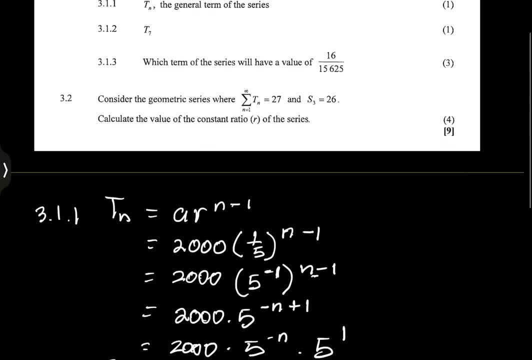 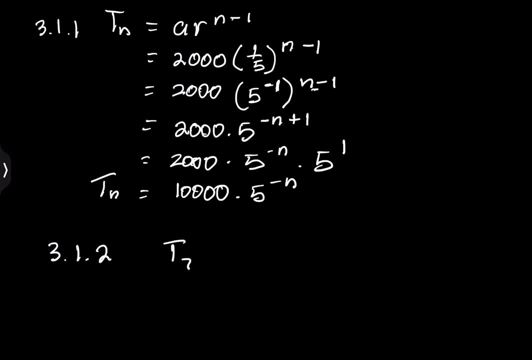 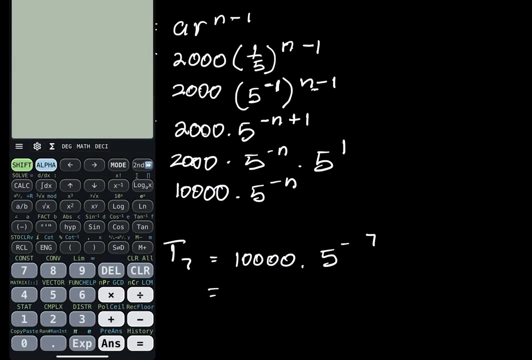 they say: well, determine the seventh term, t7. so that becomes simple once we've now simplified that. so t7 in this case would simply be ten thousand. okay times five minus, uh, seven, right, and in this case all we need to do is just take out our calculator for that. 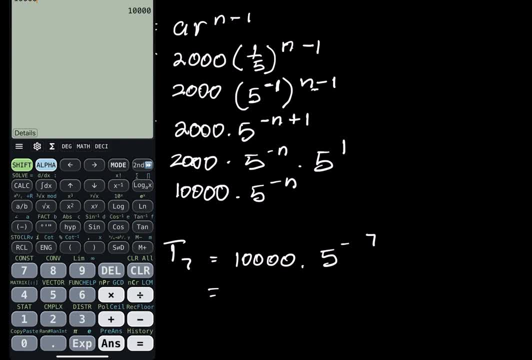 okay, so we're going to have ten thousand multiplied by five, uh, raised um to the minus seven. okay, all right, and i get an answer of 0.128 and, of course, if you want to, uh, you can express this in decimal. you can express this in decimal. 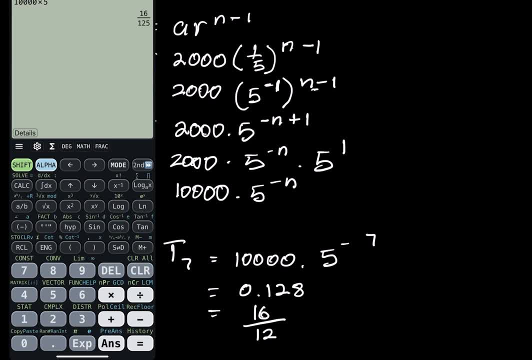 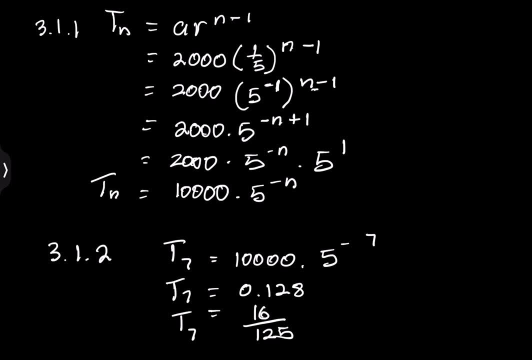 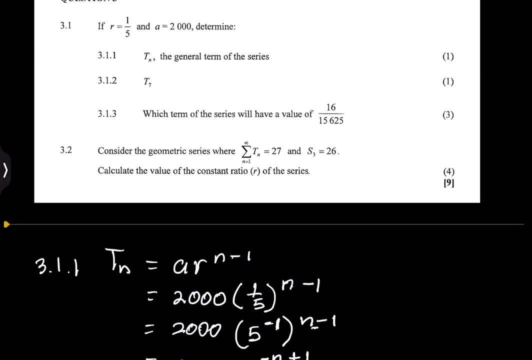 you can express this in decimal, in fraction form rather, which is 16 over 125. most likely, if you are using your casio calculator, you're going to get this answer in fraction form, and so that would be our final answer. all right, now let's go on to the next question. they say which term of the series will have the 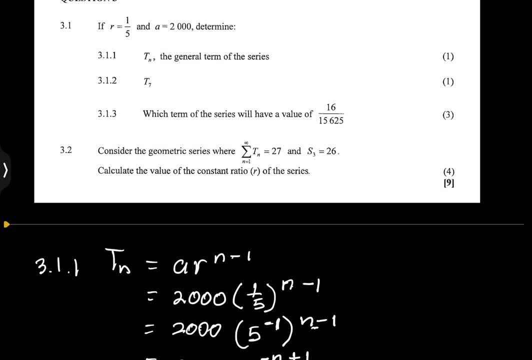 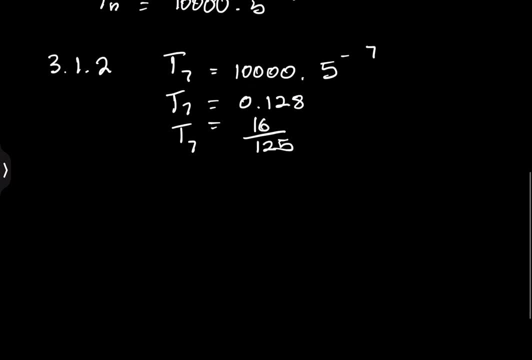 value um 16 over 15625, 15625, okay, so. so now we want to find out. so, 3.1.3, i believe. okay, right, so we want to now find out which term of the sequence of the series um will have. um will be equal to that whole number there. so i've got. 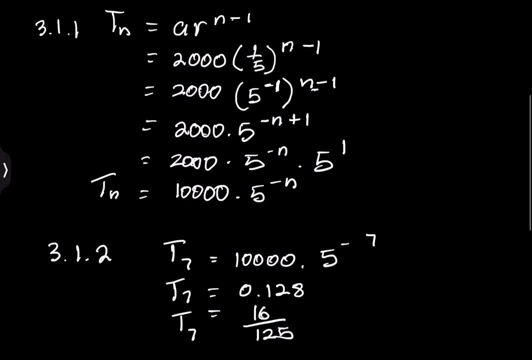 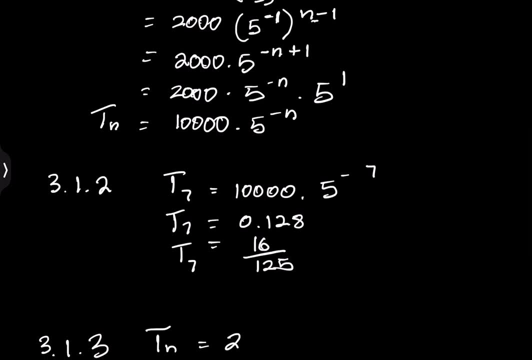 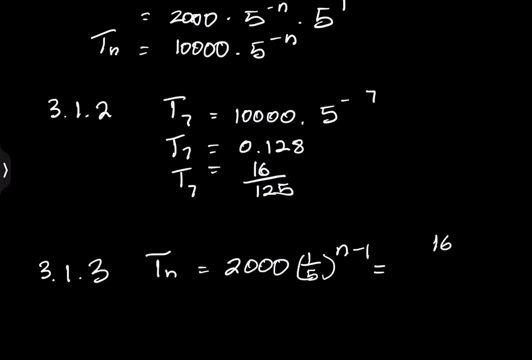 um, and, and if you wanted to write it in the original format, uh, maybe i'll keep to that. okay, um, um. so we had two thousand uh multiplied by uh, one over five, okay, to the n minus one, okay. and we said this would be equal to sixteen divided by uh. if we note this, fifteen thousand six hundred and twenty. 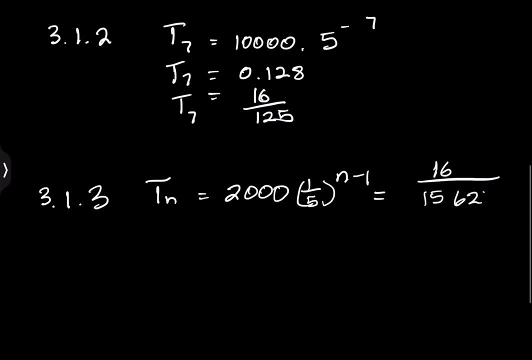 five, okay, six hundred and twenty five. so in this case now, um, i honestly would have preferred the, you know the, the initial way in which we had written this down. okay, um, so we said: this is actually the same as ten thousand and multiplied by five, to the power minus n right. and in this, 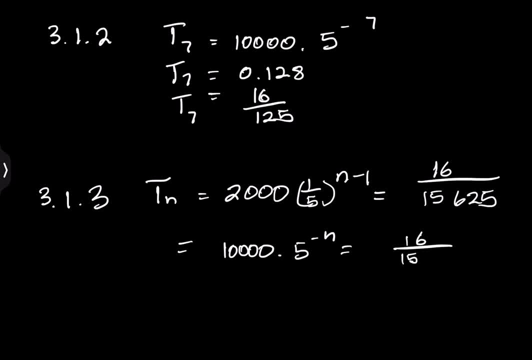 case, it would give us that 16 over, uh, fifteen, six, two, five, all right now, this is not, uh, really clear to us, um, in terms of you know which which it might be. so in this case, we can divide 10 000. okay, uh, what i do on the left, i do on the right, so this would be the same as multiplying by. 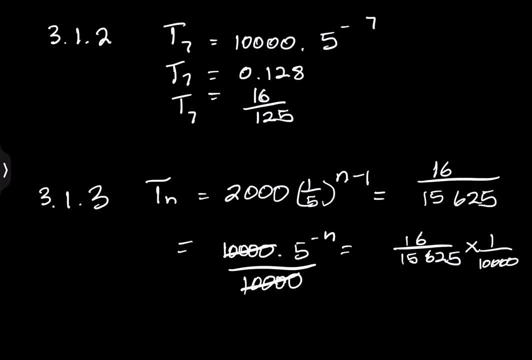 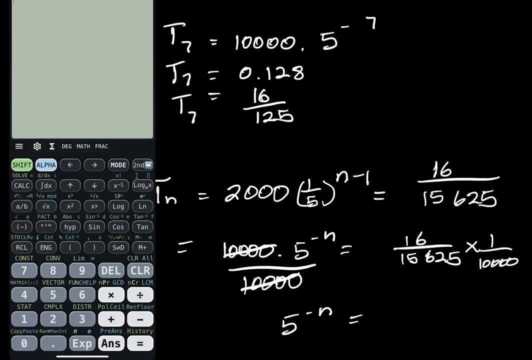 1 over 10 000. okay, that cancels with that. so 5 to the power minus n. okay, so let's do that quickly. um, so we've got 16, uh over 15 625 and we are dividing that, so let's do this, okay, so this is. 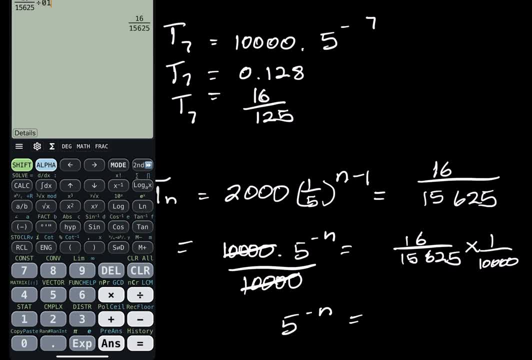 divided by, uh, 10 000. okay, so 10 000 and we get that whole number there. okay, so now, uh, what we're going to do. so this is 1 over 9765625. okay, so all i'm going to do just to make our work a little. 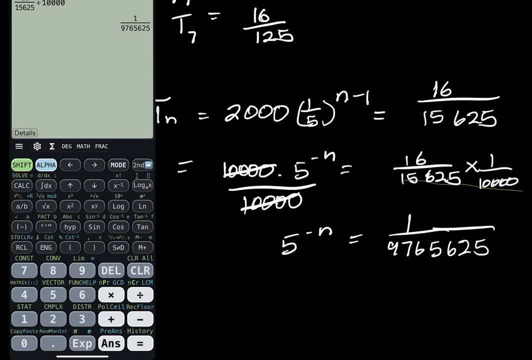 bit easier. let's just introduce logs here, right, um? so all that i'm simply going to do is look, um, if we introduce logs, then i'm going to say: well, the log of five to the minus n would be equal to log of that whole number 1 over 9765625. okay, right now. 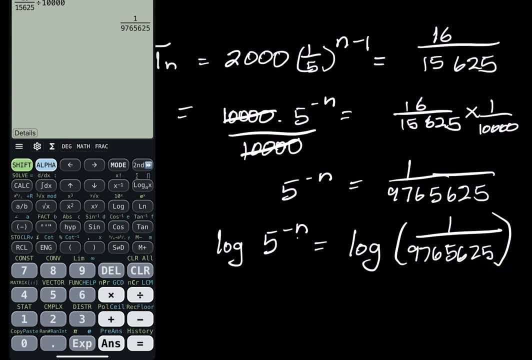 remember, when it comes to logarithms and we say the power, we jump down, okay, so that's minus n log of five, okay, which is equal to the log of that whole thing. now i'm simply going to take that number and i'm going to take the whole number, and i'm going to take the whole number. 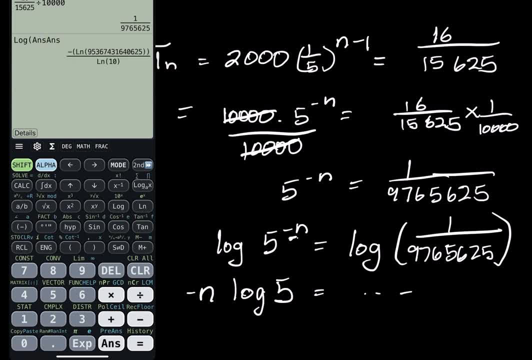 and just take the logarithm of our answer. uh, yeah, there we go. uh, the logarithm of our answer, right, um, and i get that whole complicated thing over there and divide by uh, the log of five: okay, log five, okay, i get minus 10. so in this case, um, remember, we had that whole answer on the. 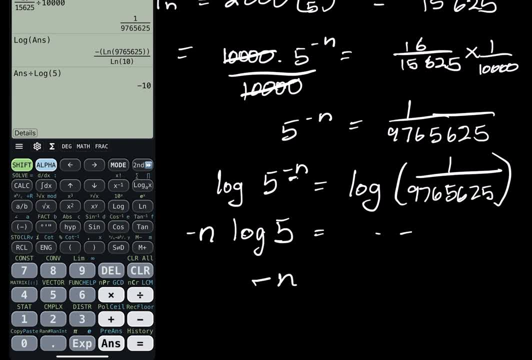 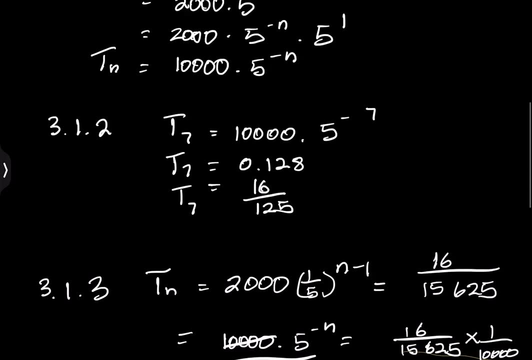 left hand side. so we're going to divide by the log of five and we're going to divide by the side. so it means that minus n is equal to minus 10, and so n is therefore equal to 10. so it means that the 10th term would be actually equal to um, that whole fraction there. all right, now let's go. 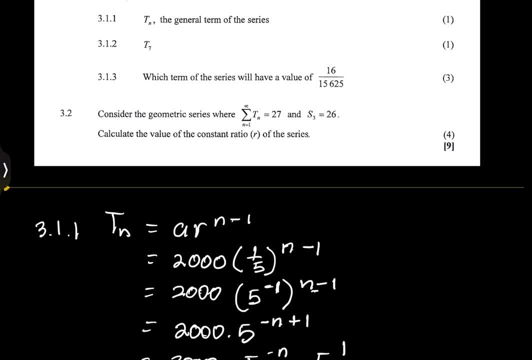 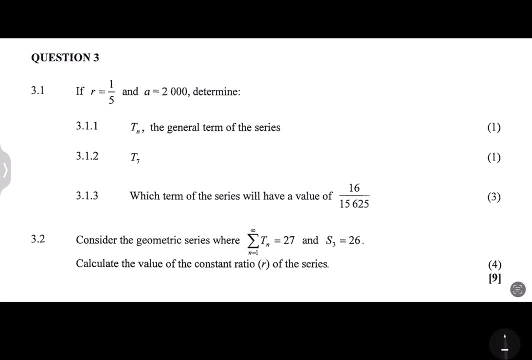 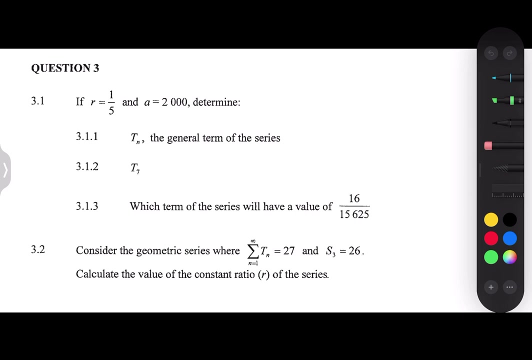 on to the next question. okay. so they say to us: um, consider the geometric series where the sum, okay. so note that um, this symbol here means the sum, okay. so where they say where the sum to infinity. so in this case we'll look at this over here and we know that they're talking about the sum to infinity. 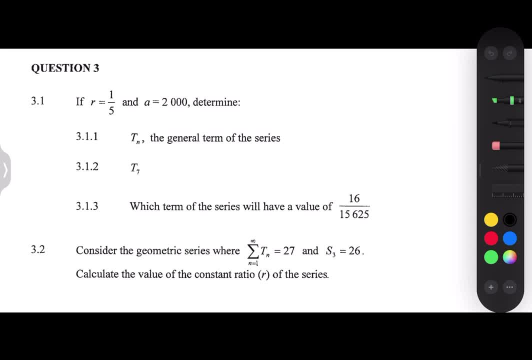 okay, so what they're simply saying is that the sum to infinity of this is actually 27, right, and then the sum of the first three terms is 26, so we're going to have to, um, and, by the way, the fact that our ratio is uh, um, we've got a sum to infinity- means this must be a, a convergent. 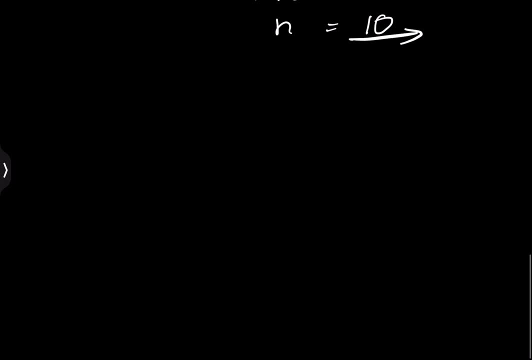 sequence right where r is between minus one and one. so, um, so what we're going to do is: so we know that the sum to infinity in this case is simply a over one minus r. okay, they said: this is equal to 27. okay, so they're going to do this, and they're going to do this, and they're going to do this, and. 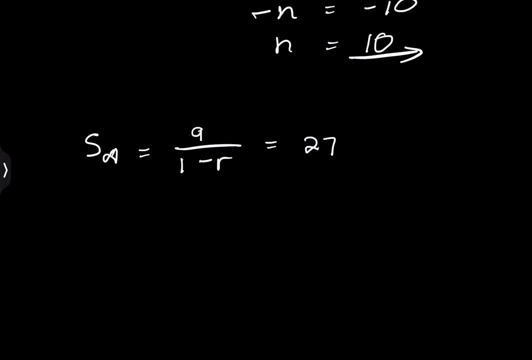 they only told us we don't know what the value of a is. we don't know what the value of r is, the common ratio. but they also said the sum of the first three terms- okay, and we know how we express this- is a to the one minus r to the power n divided by one minus r. now remember our n value. 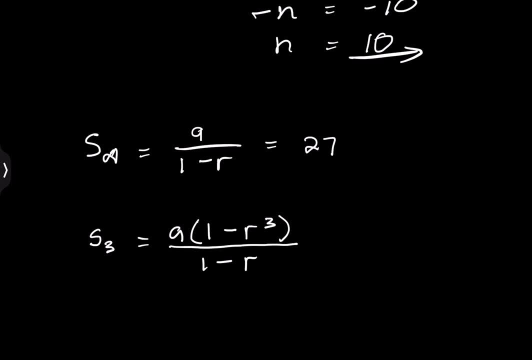 is three, so i'm just simply going to substitute that there. okay, and they said this is equal to 26. sorry, um, so that's 26. so what i'm going to do? um, let's call this equation one and let's call that equation two. so, from equation one, what i'm going to do is i'm going to make a. the subject: 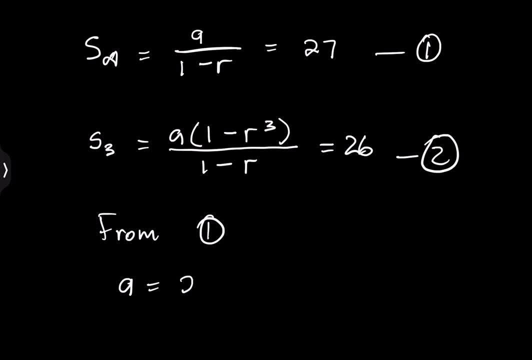 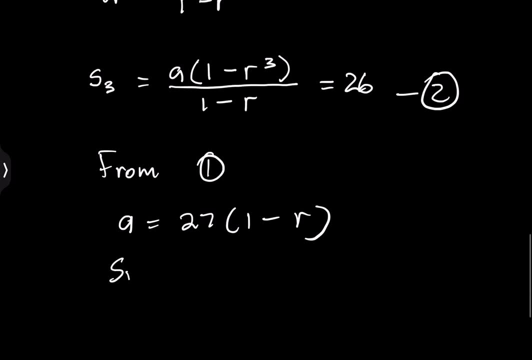 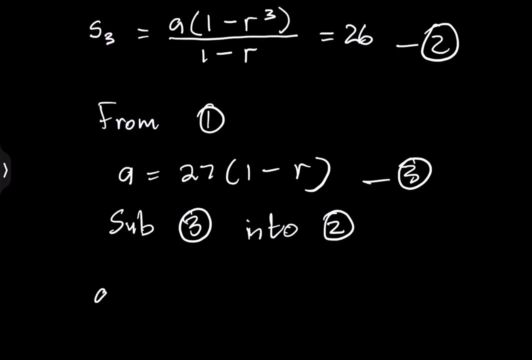 of the formula- so a is equal to 27- into one minus r. so then i'm going to substitute equation- let's call this equation three. so substitute equation three into equation one. uh, equation two, rather um. so uh into equation two. so, um, right, so what i'm simply going to do is uh, where there's a in my equation two, i'm going to